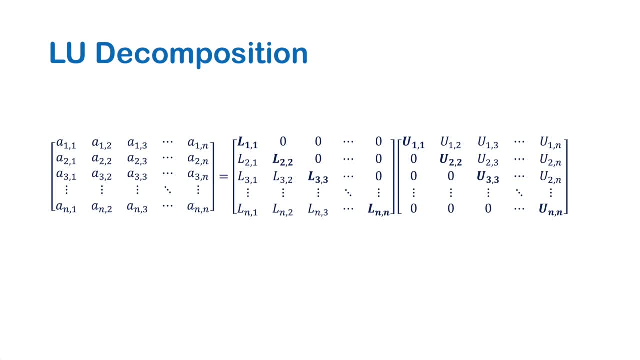 matrices and the methods used to get them are called the LU decomposition methods. In these methods, a given matrix of coefficients a is resolved to two square matrices of the same size. The first is called the lower triangular matrix, which all nonzero elements lie on and below the main diagonal. The second 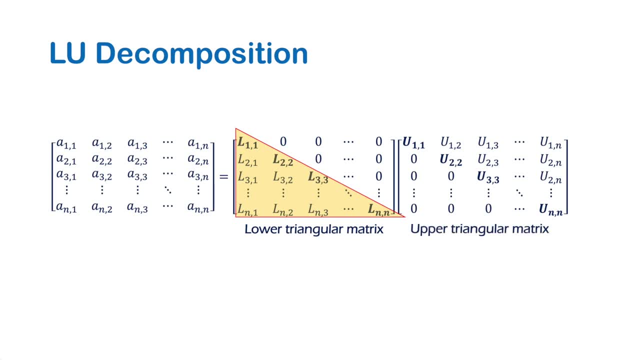 is called the upper triangular matrix, and it has all nonzero elements on and above the main diagonal. This operation can be written in a simpler notation, such as that: the matrix A is equal to the inner product of L and U. You should remember here that the matrix multiplication is not commutative, which 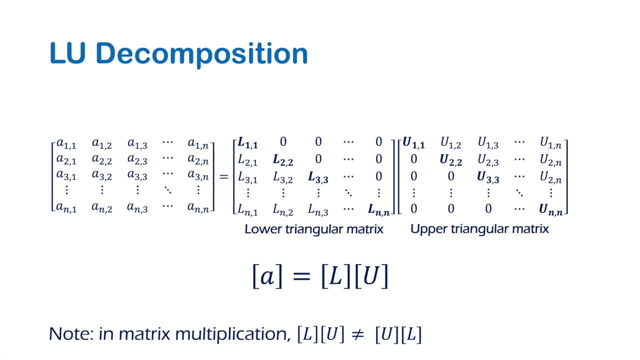 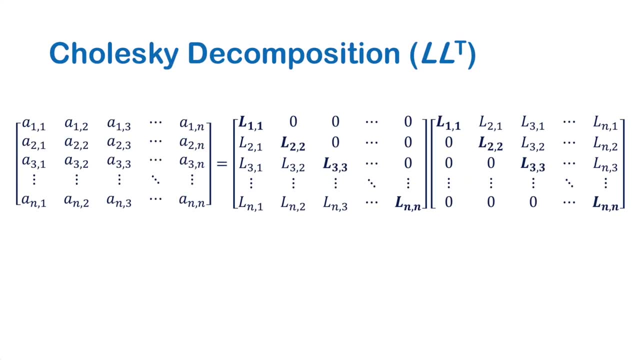 means L multiplied by U is not equal to U multiplied by L. Cholesky decomposition, or as more known as Cholesky factorization, is a method applied to the matrices with special conditions. First, the matrix should be symmetric. Second, it should be positive. definite: The condition of symmetry makes the computation. 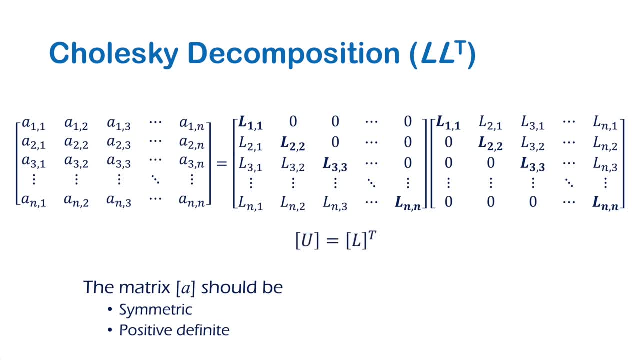 of the lower triangular matrix. enough for factorization, because the upper matrix is simply the transpose of the lower matrix. Consequently, the components of the matrix A will be L multiplied by LT or L transpose. The two requirements or conditions of Cholesky factorization must be satisfied before. 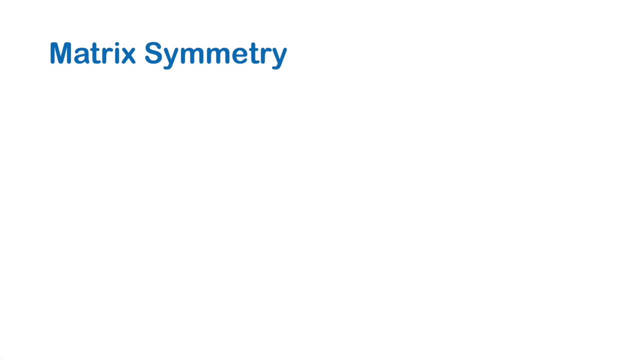 applying the method. First, let's speak about the symmetry. The matrix is described as symmetric if it is a square matrix and the elements are mirrored above the main diagonal. This can be represented by using element indices, as A Hij is equal to A Ji for x, for y, for y, for e. In other words, this means: 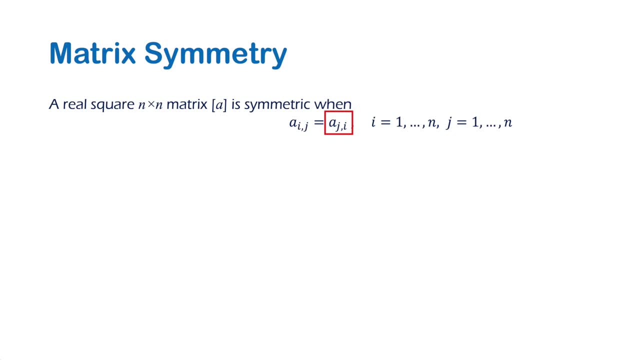 that the matrix has a critical value that is closer to the boundary of the coordinate. all i and j, For example. this matrix is symmetric because every element about the main diagonal is reflected below it. Let's check some elements. a12 is equal to a21,, which are equal to 0.. a23 is equal to a32,, which both are equal to. 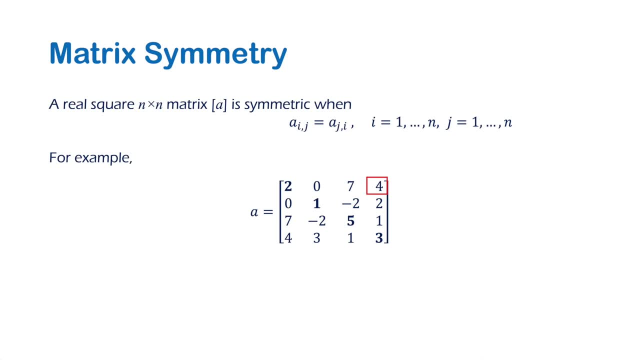 minus 2, and a14 is equal to a41, which are both are equal to 4, and so on. Therefore, it's obvious that a symmetric matrix should be equal to its transpose, A real matrix. A is positive definite if the product of its. 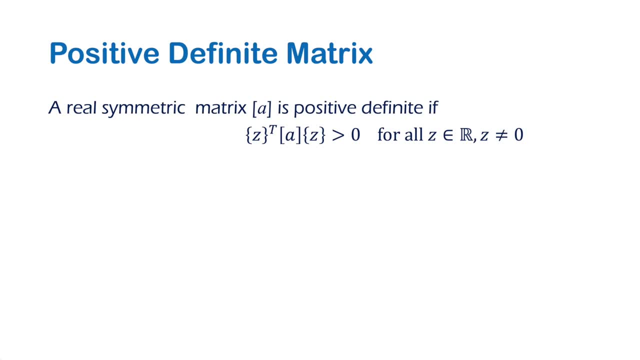 multiplication from the left side by a vector Z- transpose- and from right side by a vector Z- transpose. vector z is always positive for all real number of z except 0. This is a mathematical definition. Let's see an example. The identity matrix is positive definite. So if we carry out the 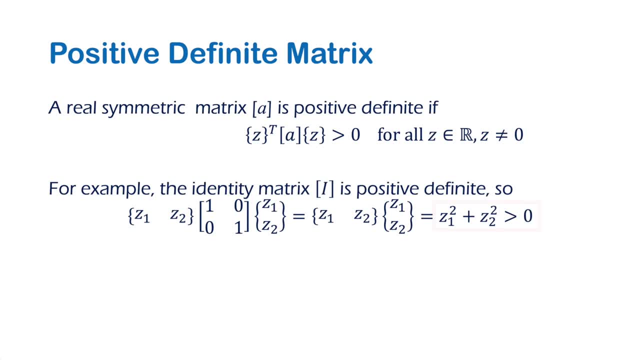 multiplication shown here, the result will be z1 square plus z2 square, which is always positive for any real value of z1 and z2 except 0.. The method of vector matrix multiplication shown here is not practical to test whether the matrix is positive, definite or not. An easier way- 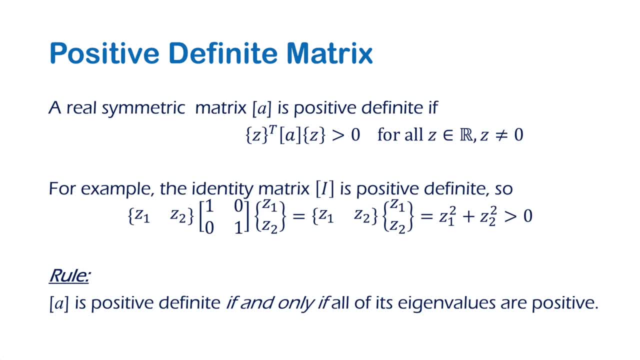 is to apply the following rule: A matrix is positive, definite if, and only if, all of its eigenvalues are positive. So the definiteness of a matrix can be tested by using eigenvalue functions of z1 square plus z2 square. The matrix is positive, definite if, and only if, all of its eigenvalues are positive. So the definiteness of a matrix can be tested by using eigenvalue functions. 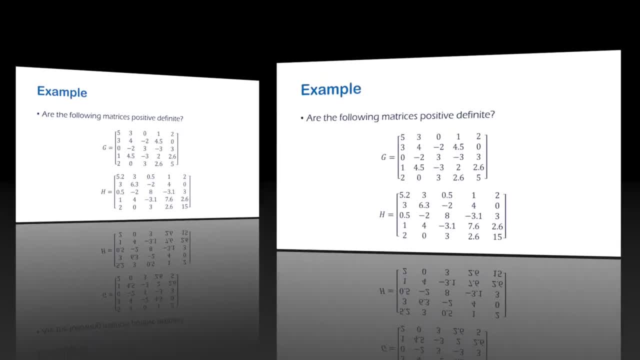 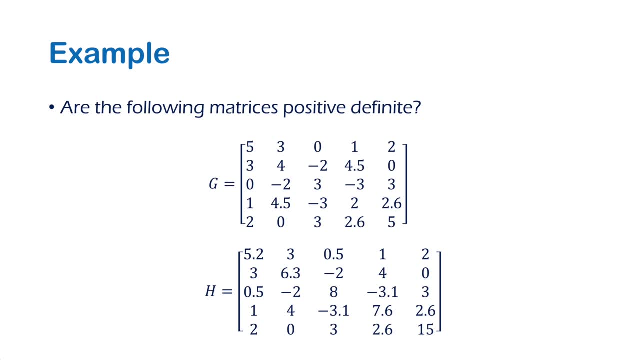 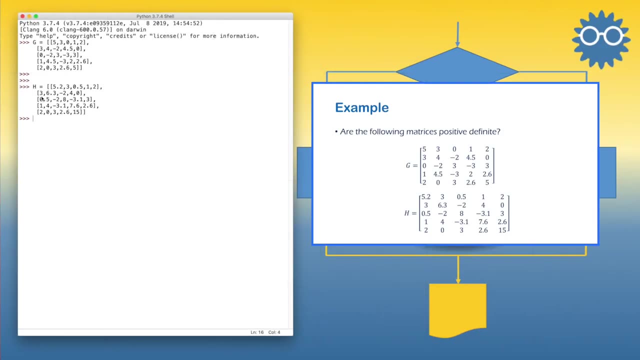 from the linear algebra module of numpy. In this example, I will show you how to use the functions of eigenvalue in numpy in order to test the positive definiteness of the matrices g and h. As you see, here we have defined the matrices g and h, So now let's test each matrix. 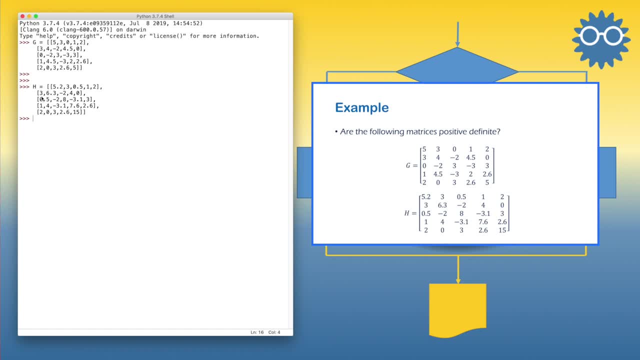 for positive definiteness. So first we can use the, let's say, import. then this function returns the eigenvalues of a given matrix. So let's test the g matrix. See, we have the eigenvalues of the g matrix and, as you see, all elements are positive except number four or the fourth element. 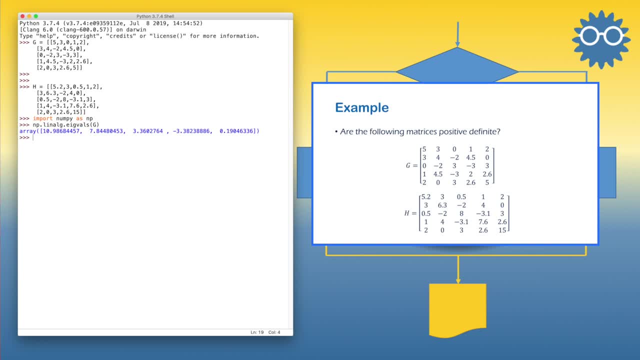 which is negative. So that means we cannot decompose this matrix by using Cholesky decomposition method. We can use another function. This function is more comprehensive than the first one because it returns both eigenvalues of the matrix, eigenvalues and the eigenvectors. So, as you see, the eigenvalues are the first. 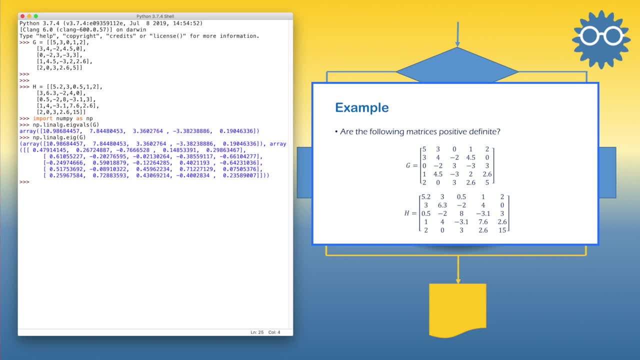 row of the output In order to get the first row only. we can make simple trick here Now. this shows that we have a tuple of V and underscore, because we don't need the matrix of eigenvectors, so that's why we assign it to the underscore, while if we try to return the value of V, we get the eigen. 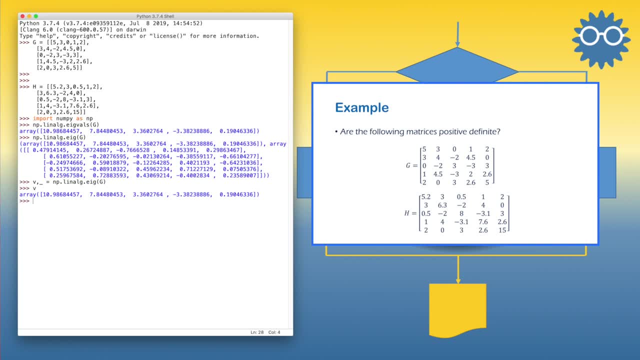 values of G, and, as you see, it's the same result. Now let's test the matrix H, so we can say: by the same way: lean, the all values of the eigenvector of the matrix H are positive. so that means this matrix can be decomposed or factorized by using: 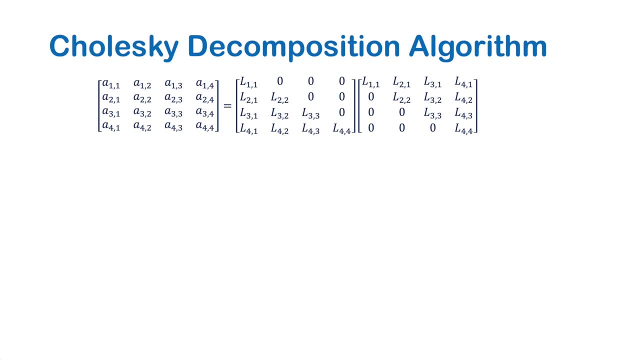 Cholesky's method. The algorithm of Cholesky factorization can be developed simply by multiplying the symbolic components L and LT, then equating each algorithm by simply making two algorithmically mirrored, say unit snap: 그랬肩astre: the Salix' scale and the logic field. the parameter space stripe is also a 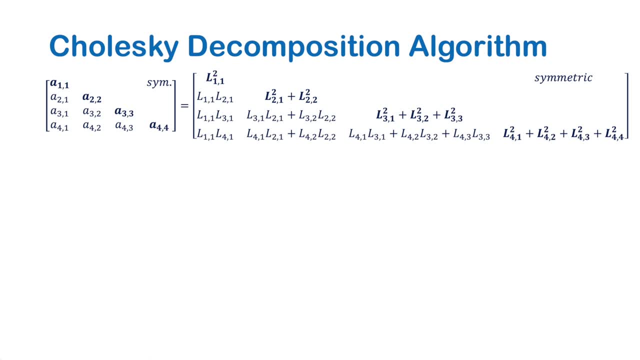 element in A with the corresponding element in the product matrix. as you see here in this 4x4 matrix, Because both matrices are symmetric, the algorithm can be formulated by using the elements in the lower triangle. The formulation goes column by column, so 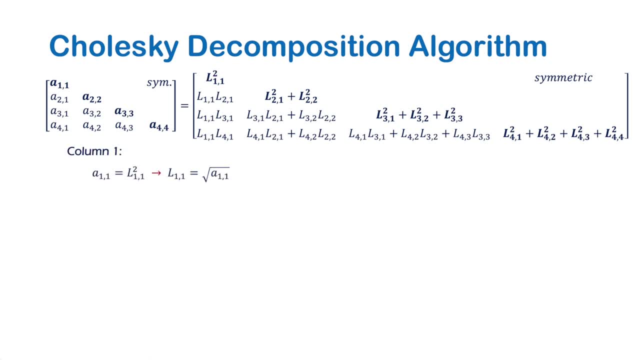 we start with the column 1.. First we get the element L11, then L21, which is calculated using L11.. The same thing is done with L31 and L41.. The elements of column 2 of the lower matrix can be found by using the calculated elements in column 1.. The element L22 is found. 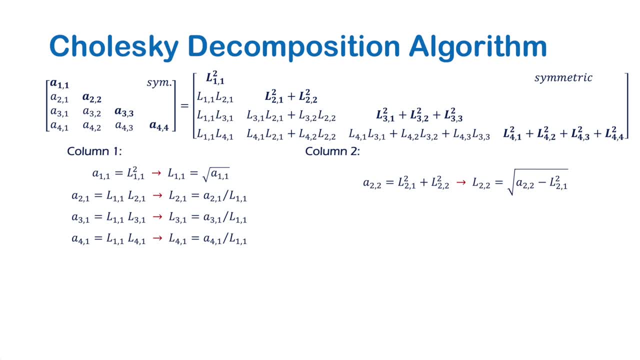 by using A22 and L21 from the first column and second row, L32 is found by using A32, L31 and L21.. L42 can be found also in the same way. Similarly, the third column can be found in the same. 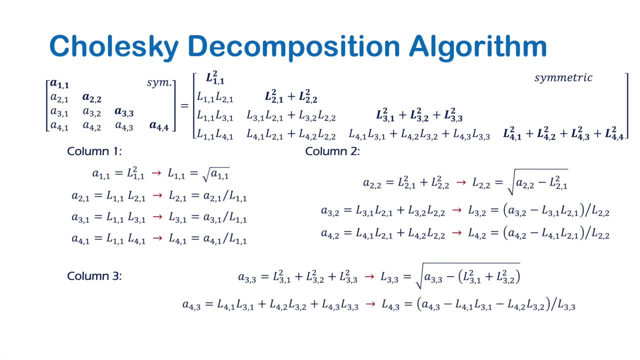 way by using the elements of L from the previous two columns and so on. The last column should have only one element on the main diagonal and, as you see, it is found by using all elements in the last row found before Now by close looking to the indices of each element in. 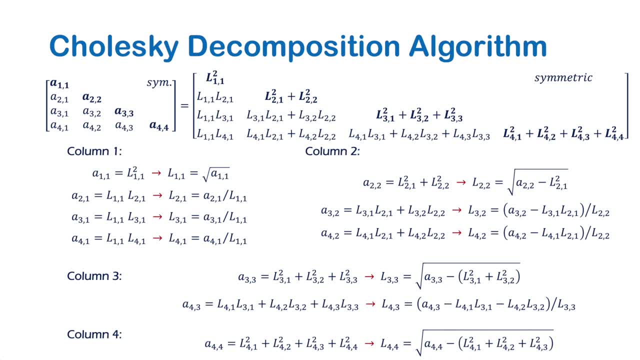 this formulae we can find the general pattern of each row and column. For example, the L2 terms and the calculations of L22,, L33 and L44 have the fixed index of the rows, while the second index, as you see here, goes from 1 to the number of rows minus 1.. Similarly, 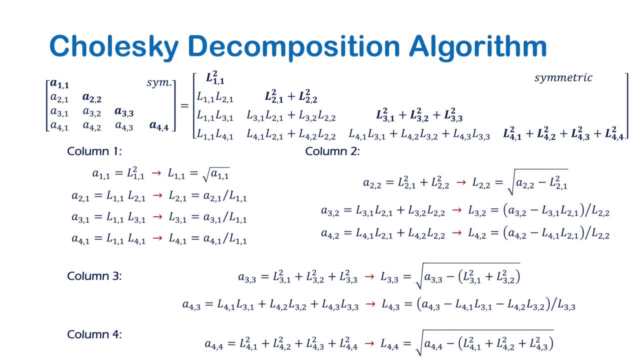 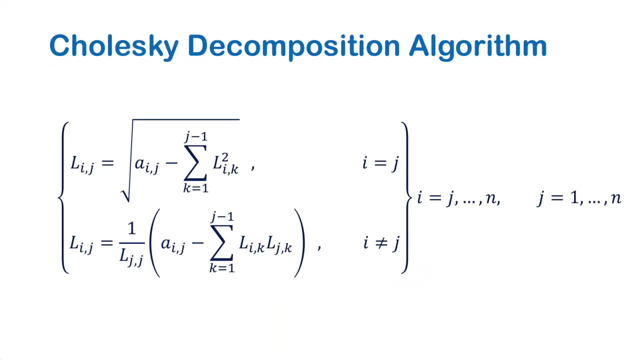 patterns can be seen in other elements with different row and column numbers. That helps us to write the general formula of Cholesky's algorithm. The algorithm consists of two elements. The first is the column 1,, the second is the column 1.. The second is the column 2, and the third is the column 3.. All these are the same The. 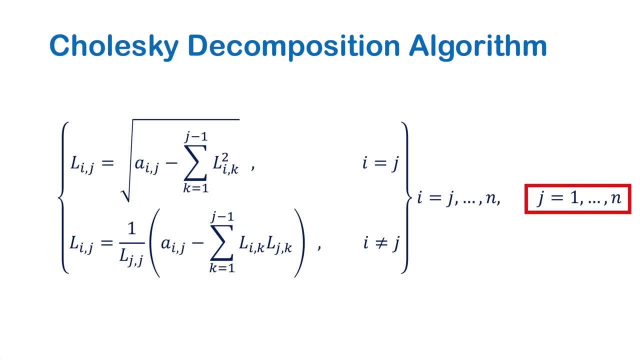 two nested loops. The J loop is the outermost loop and it goes through all of the columns, since the calculations, as I told you before, should precede column by column. Next, the I loop starts at row J to compute the elements on the main diagonal and the lower ones. The first formula: 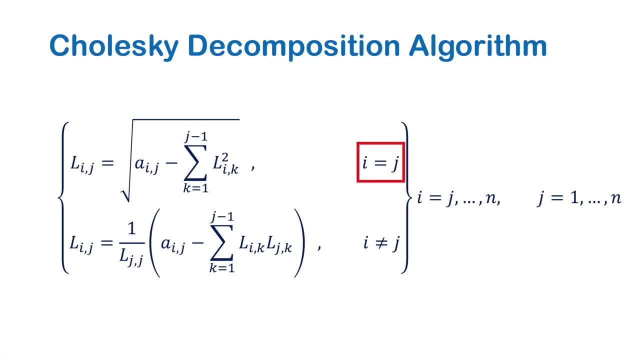 is for the elements on the main diagonal, where I is equal to J, while the second formula is for the elements beneath the main diagonal. Each formula requires an internal loop for summation. This can be done by utilizing a K loop or by using numpy sum function, with slicing as I'll. 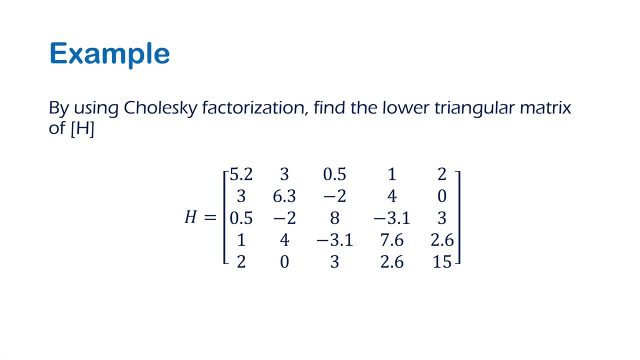 explain during the coding. In this example we have the matrix H, which we have proven that it's positive definite. But for comparison I will try factorizing the matrix G2 and show you the results. So let's go to the editor and start. 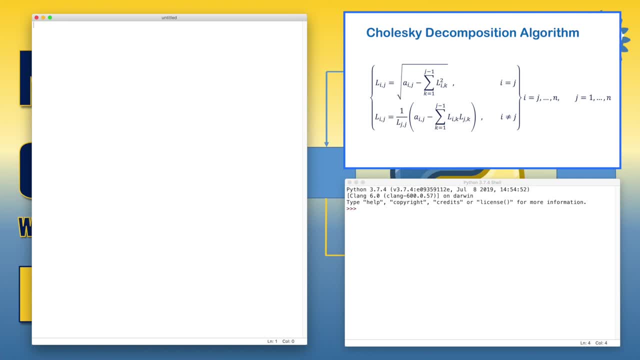 So let's start coding. So we begin by importing numpy module. Then we define the function Cholesky with one argument, which is the matrix A, where A is a numpy array. Then we define the function Cholesky, which is a numpy array. 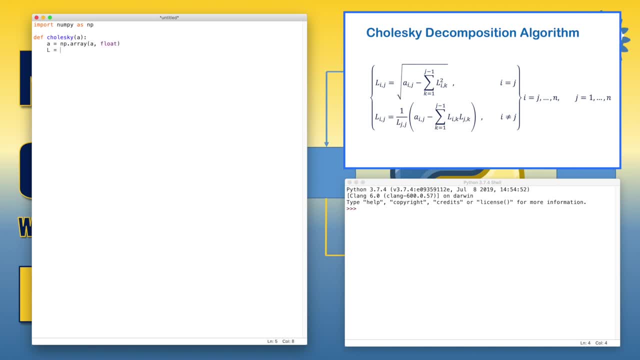 Then we define the lower triangular matrix. This function constructs a zero's matrix or zero's two-dimensional array and the same size of A. Now we need the size of A. We can use the function shape, Since A is a square matrix. so it's enough to know the value n, which is the number of rows. 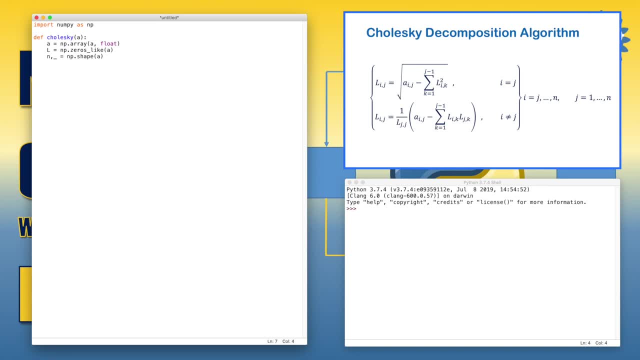 Now we start the loop of columns, Then the inner loop. Now we have two. formally Let's start with the first. We initialize the summation variable, Let's call it sum K, And we start inner loop of summation. So Lij. 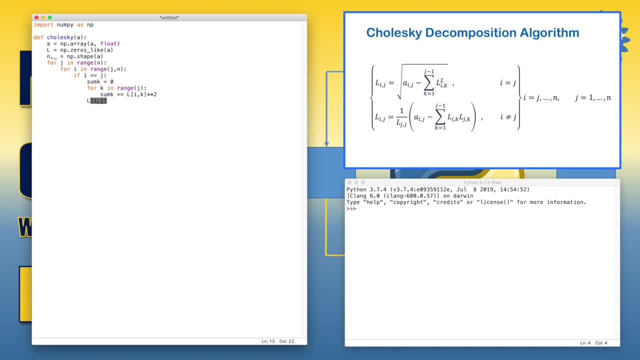 For the main diagonal element will be equal to the square root. let's go to the to write the second, so else same way. finally, we return the lower triangle. now let's test this function by decomposition of the matrix edge. in order to save time, I copied and pasted: 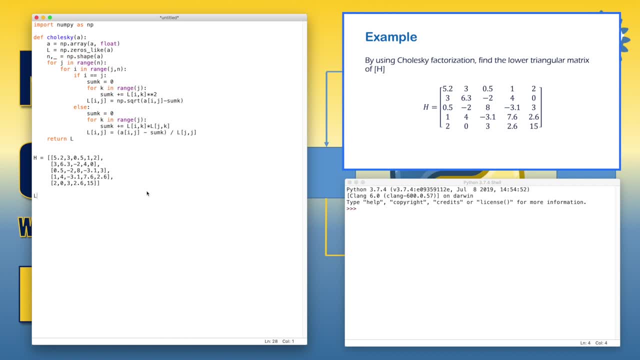 matrix edge. so let's run the function by saying that L. now, in order to verify our result, we can simply multiply this matrix by its transpose. so let's say so: MP dot is dot product function of multiplying two matrices. so the first matrix is L, the second will be. so let's, if we compare the values of the resulting 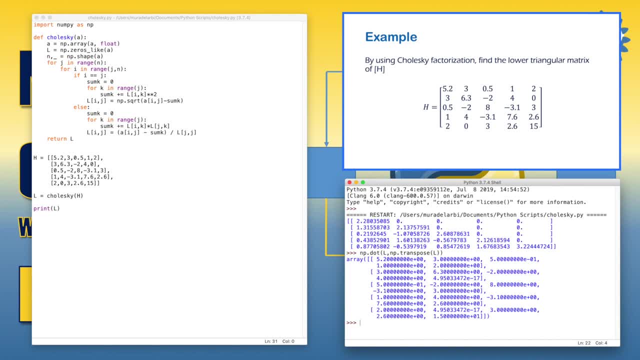 matrix, we notice that it they are the same value as we defined in in the code. so let's try G in this example. I will copy paste it in order to save time. now we define G and pass it to the argument, to the Cholesky. so let's run the code and see the result. so, as you, 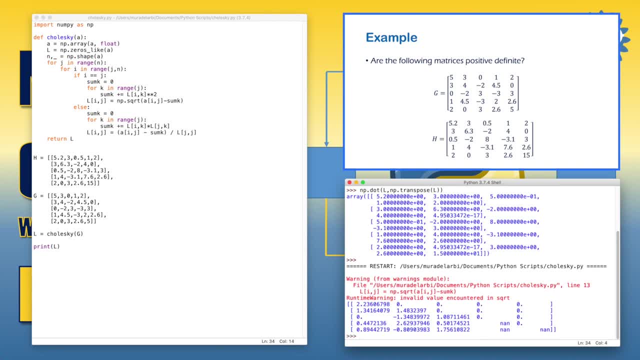 see, here we have error message or warning message due to the square root function. so that's why you will notice, if you remember, that the fourth element in the eigen values were negative, and here we see that the problem started at the fourth row and fourth column. now, before ending this video, let's use the 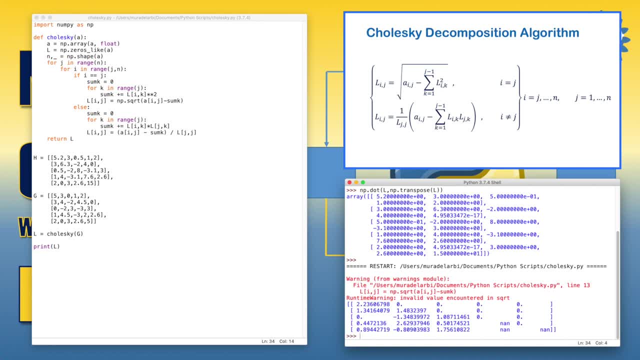 same behavior with you. we no longer have to do. the FOC satisfied that and no CHOL. and on the reverse side, we just got this fall out of place. it is quasi, because if we go back to the report we can see that my node is not dependency. 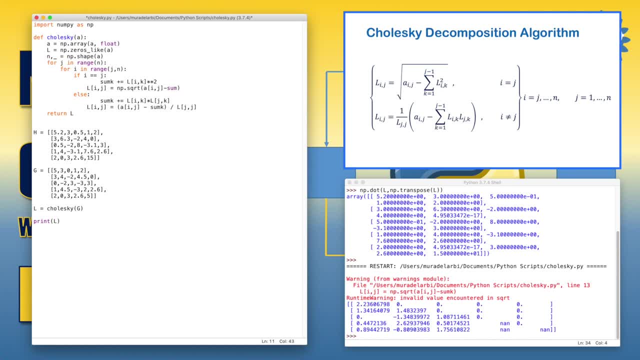 but it is showing us the call we have for the call customers with name, and we can now 선택 to reduce products that are associated with it. tesla~, but we notice something here. still, we have k, but k is a loop which goes from, let's say from: